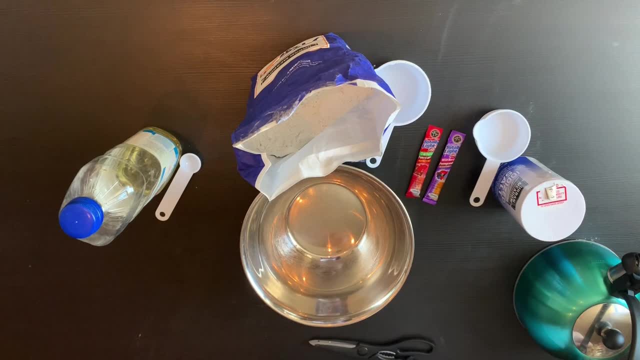 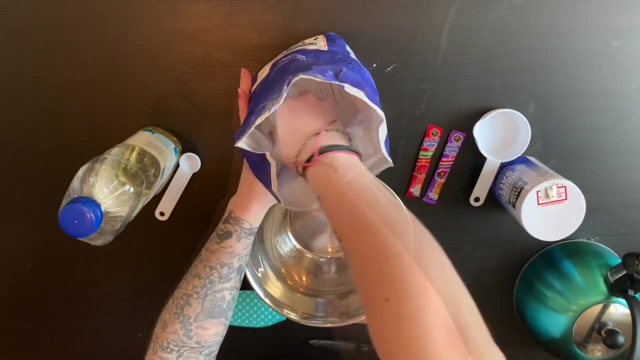 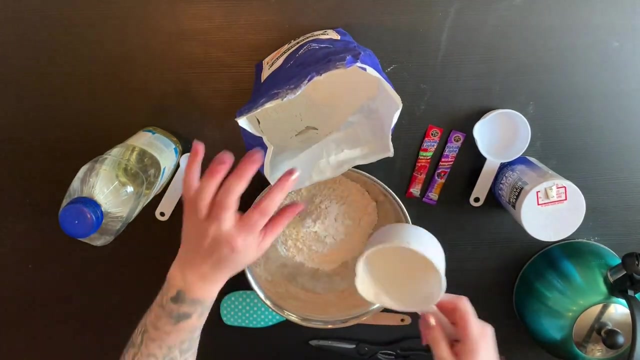 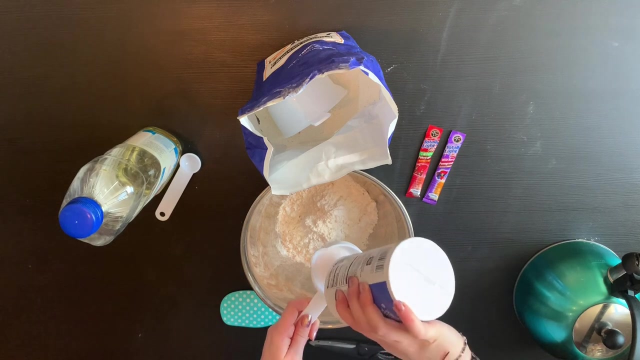 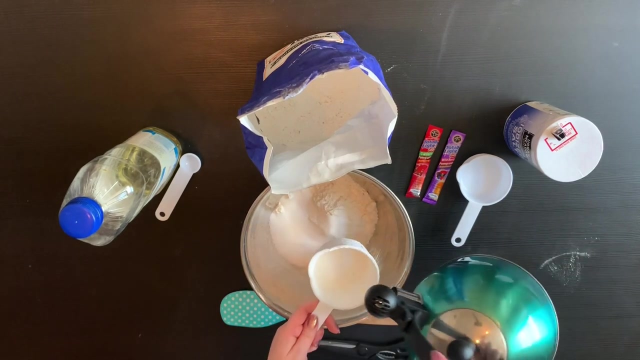 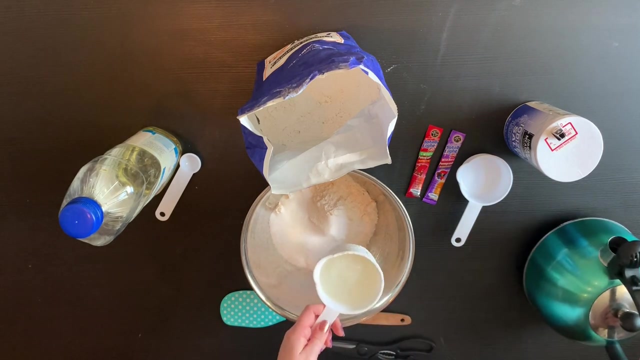 We're going to start mixing everything in a bowl to start it off with, and then we are going to go from there. So I'm going to start with my dry ingredients first. so the two cups of flour, Half a cup of salt, one cup of warm water- and this is not just super warm, like I haven't boiled it very hot- and I'm also going to add one of these coloring packets to it. 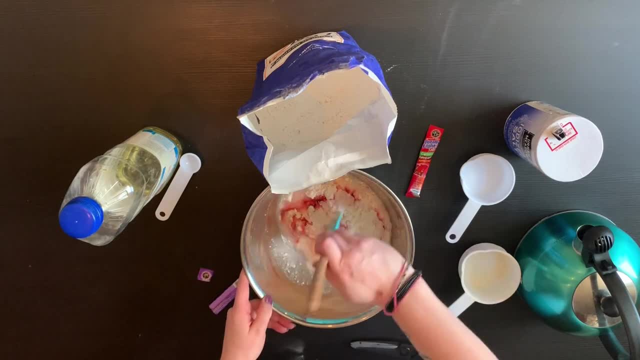 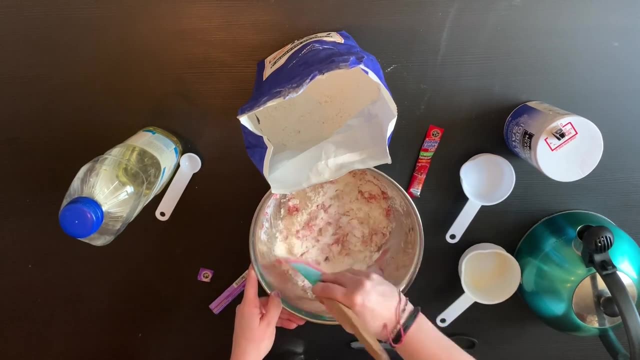 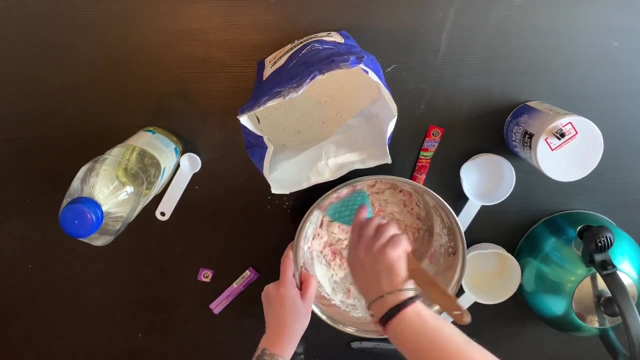 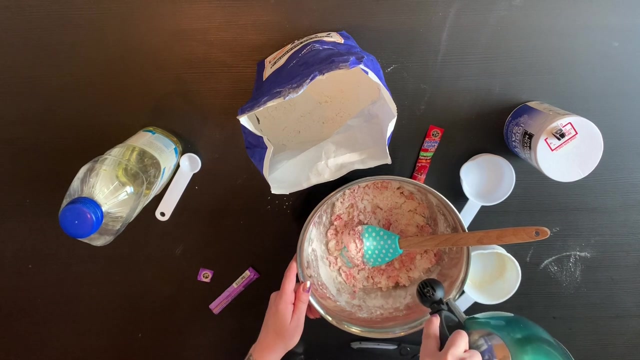 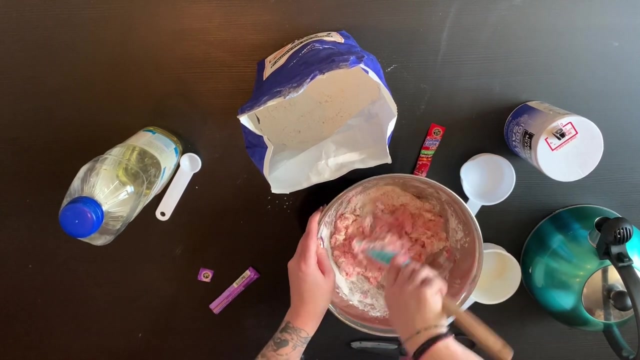 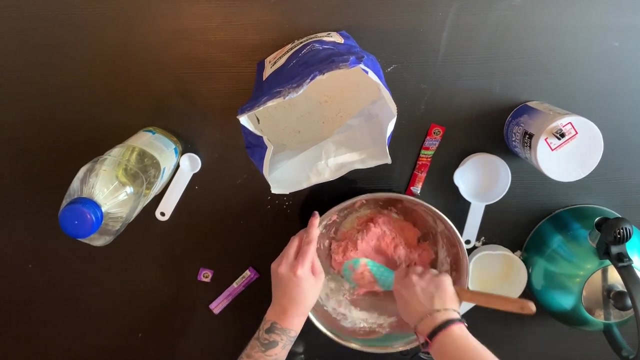 And I'm going to start by just stirring everything. This dough is a little too dry, so I'm going to add a little bit of water to help even it out a little bit, And now that this is at like a tacky point, I'm going to start kneading it with my hands. 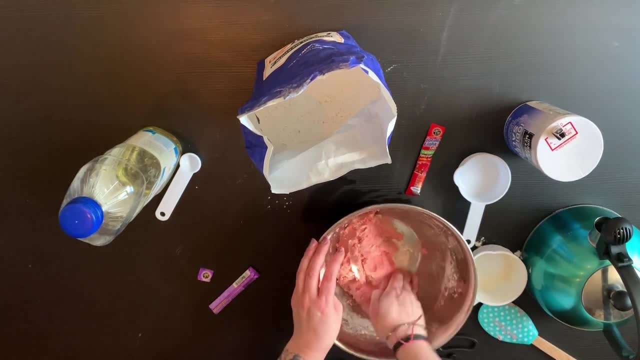 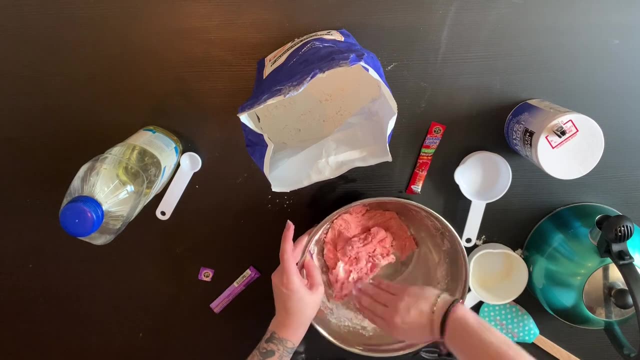 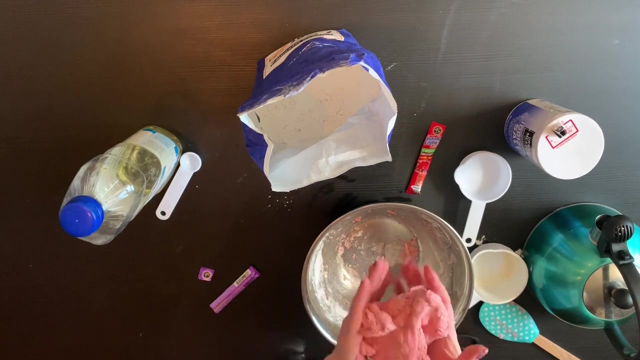 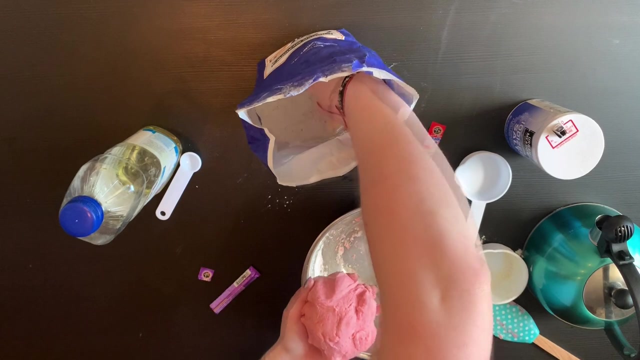 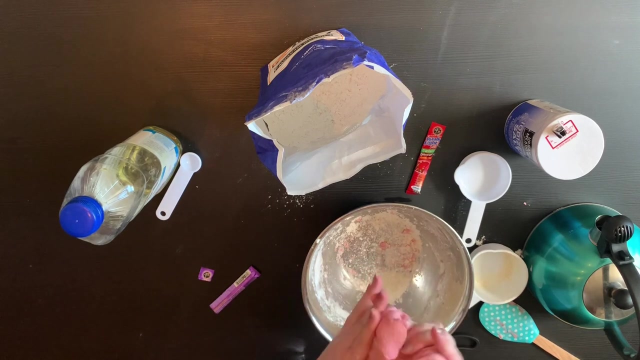 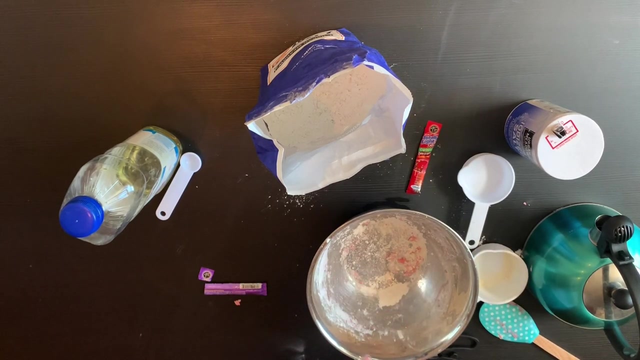 my hands. It is a little sticky at this point, so I'm just going to put a tiny bit of flour on my hands to help hold that part. Once you're at this point, you can add a teaspoon of vegetable oil on top. This will just help it with the consistency. 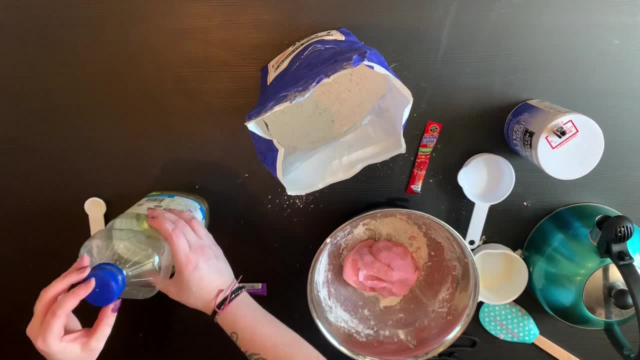 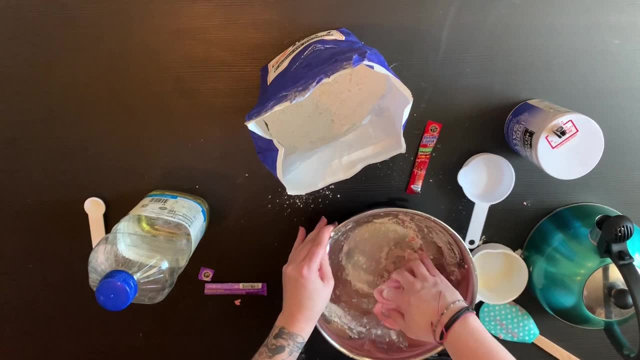 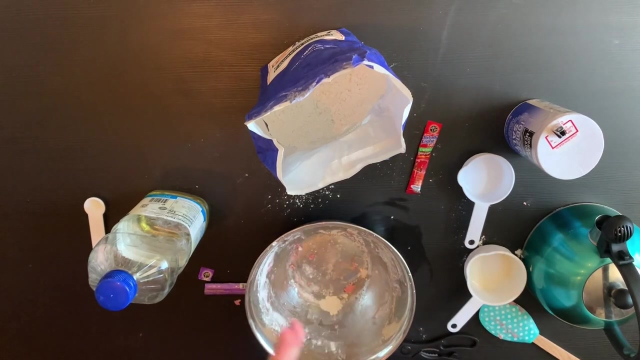 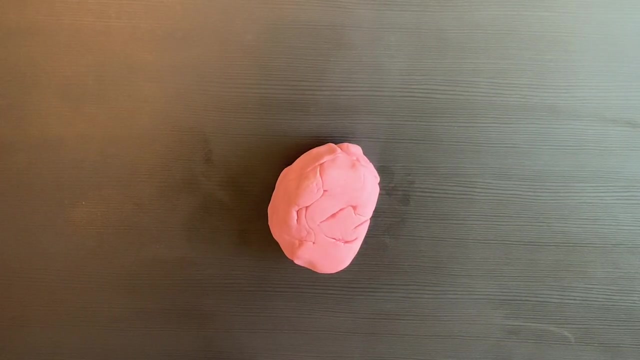 Okay. So once you've made your own salt dough- Play-Doh- it's also a really fun tool to use to practice clay techniques, So you can practice simple things like creating spheres with your clay. You can start your clay by rolling your hands counterclockwise. 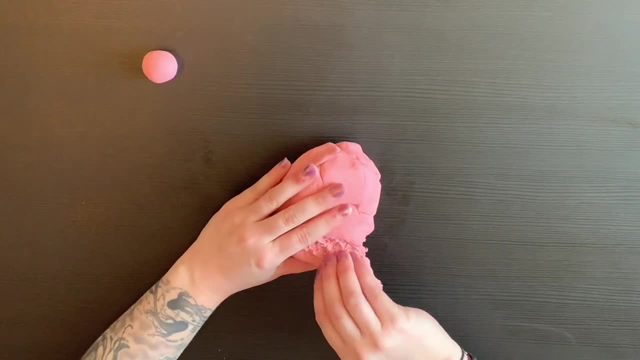 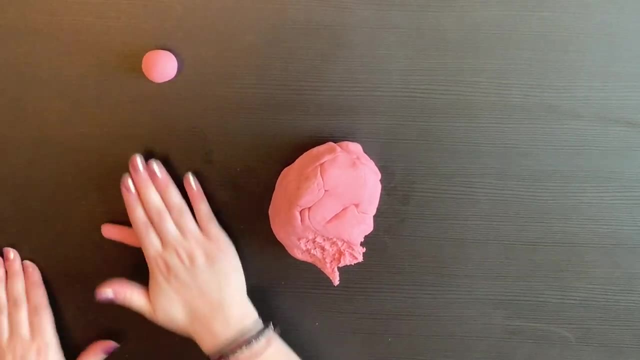 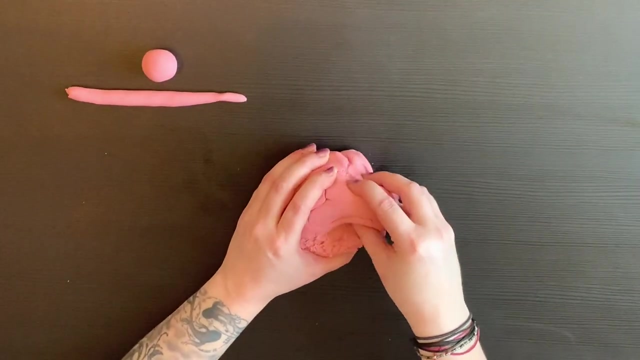 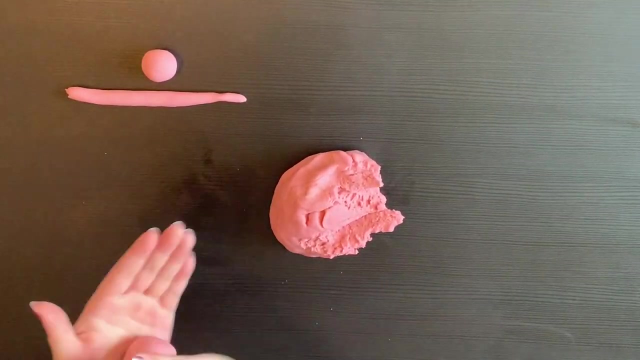 You can practice doing coils, where you rub your hands back and forth, side by side, to create almost like a snake. You can also do it with one hand on a table. You can make a pinch pot with it. So you will start with this sphere. 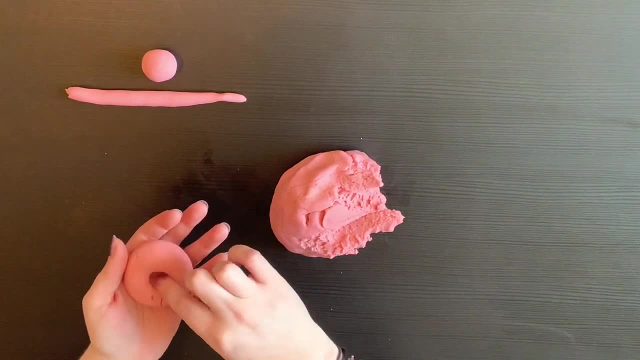 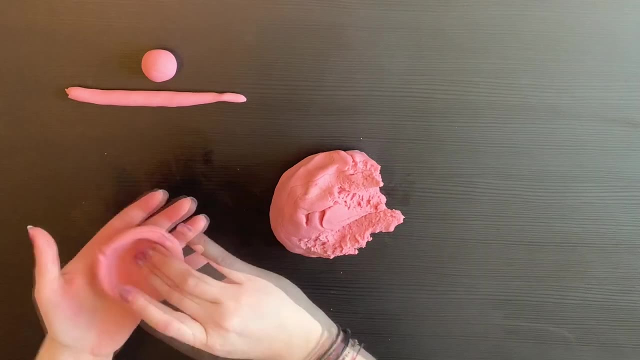 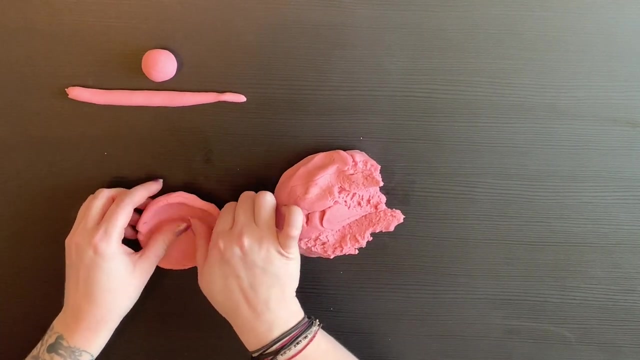 After starting with the sphere, you press one finger or thumb in And you pinch on the outside. You can press down in the middle as well to bring it out and pull. So pressing down and pulling on the wall, This will round it out a little bit more.